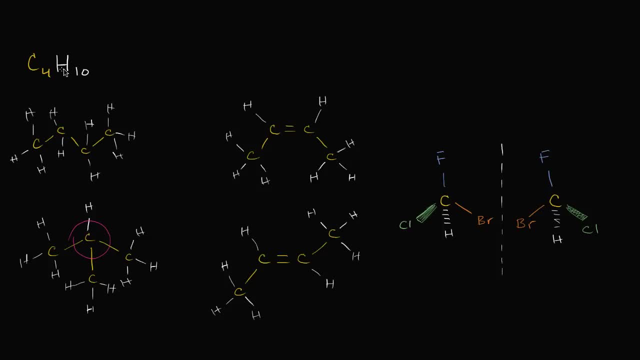 They're bonded to different things, And so when we have the situation where you have the same constituent atoms, where you have the same chemical formula, but you're still dealing with different molecules because of either how their bonds are made or what their shape is, we call those isomers. 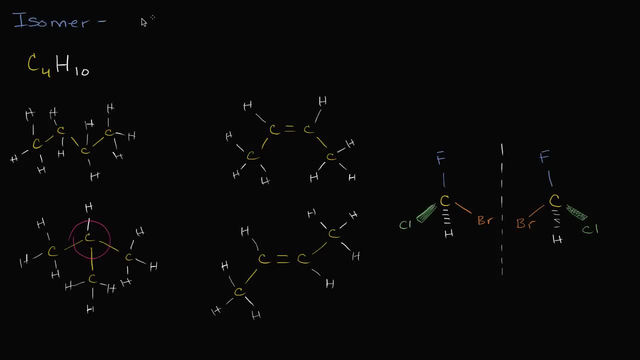 So an isomer, you have the same chemical formula But you could have different bonding, but different, different bonding. bonding or shape Bonding, shape or orientation, orientation. So over here you have just different bonding. 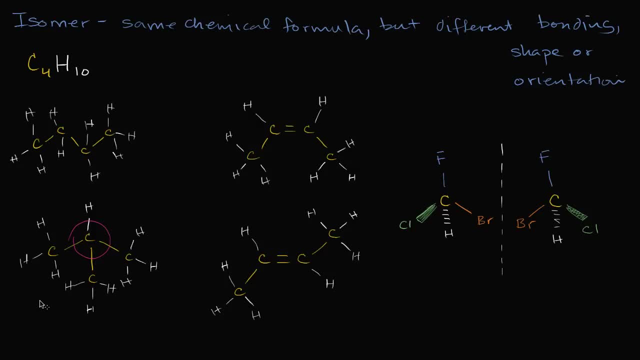 And this type of isomer is called a structural isomer. So these characters are structural isomers: Same constituent atoms, but different, different bonding Structural isomers. So that's structural isomers right over there. Now, when you look at this pair or this pair, 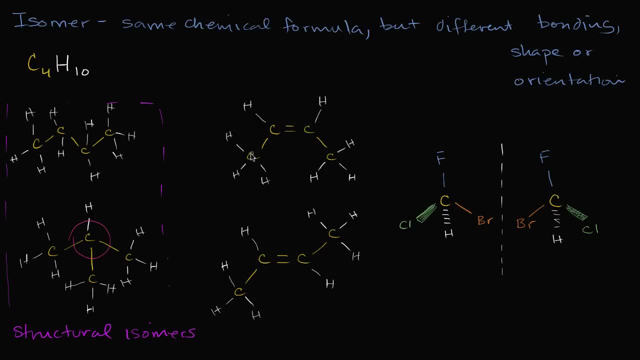 you say: well hey, those don't look like structural isomers. Not only do they have the same constituents, both of these, for example, have four carbons. four carbons, and they both have one, two, three. 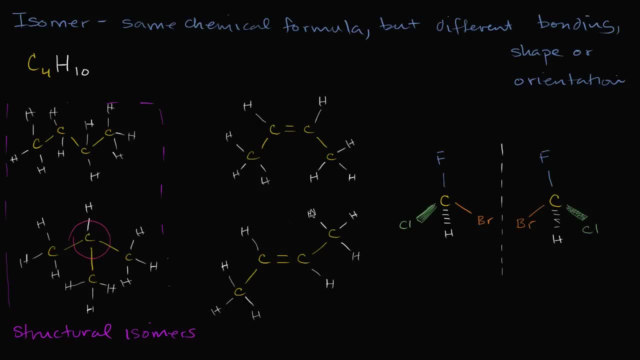 four, five, six. well, one, two, three, four, five, six, seven, eight, And they both have eight hydrogens, So we could both. these are both C4H2O, C4H2O, C4H2O. it looks like they're bonded similarly. 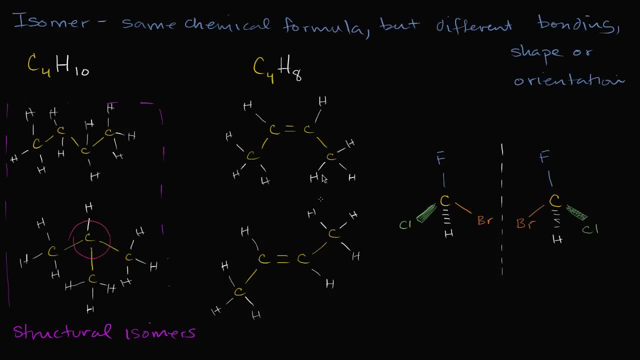 For example, I mean the left-hand side here. these look identical, and on the right-hand side you have a carbon bonded to another carbon that's bonded to three hydrogens. Carbon bonded to another carbon that's bonded to three hydrogens. 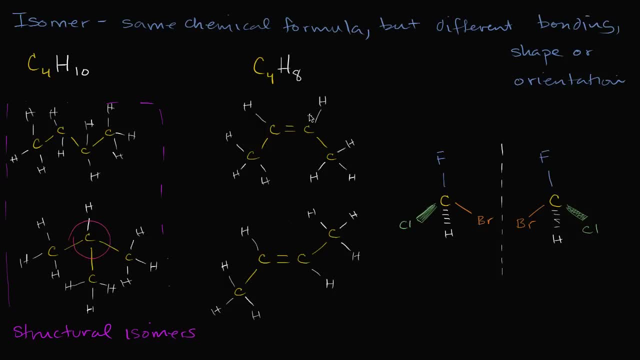 Carbon bonded to a hydrogen, Carbon bonded to a hydrogen. So it looks like the struct, the bonding, everything's bonded to the same things. but you might notice a difference Over here on the right-hand side. this CH3 is on the bottom right. 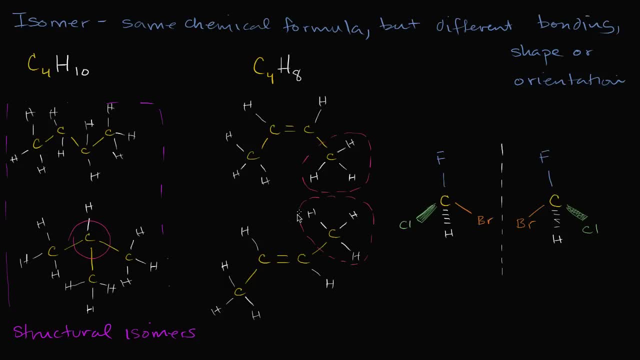 while over here it's on the top right And you might say, okay, well, you know what's the big deal there. These, you know all these molecules, they're all moving around. Maybe they're rotating with respect to each other. 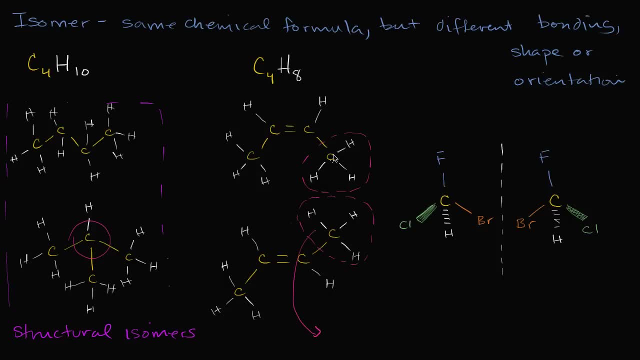 And these things could, this thing could have rotated down to become what we have up here if this was a single bond. A single bond would allow for that type of rotation. It would allow for these things to rotate around each other, for the thing, the molecule, to rotate around that bond. 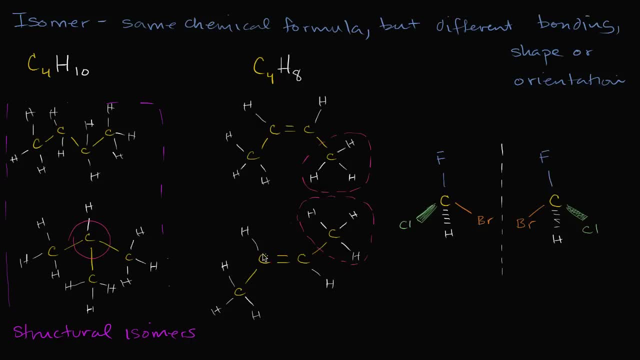 for the thing, the molecule to rotate around that bond. But a double bond does not allow that rotation. So this fixes these two things. this fixes these two things in place And because of that these are actually two different molecules. Over here on the top you have the CH3 groups. 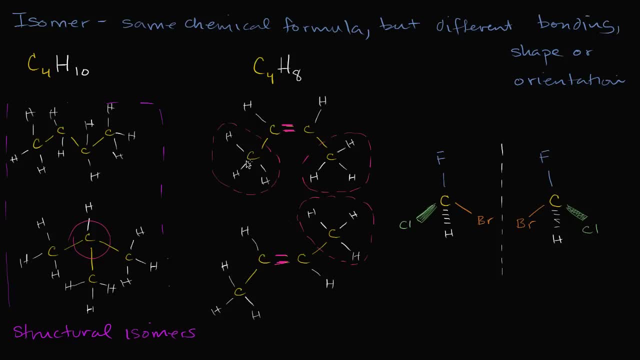 They're both. they're both on, they're both, I guess you could say, facing down, or they're both on the same side of the double bond, While over here they are on different sides. They are on different sides of the double bond. 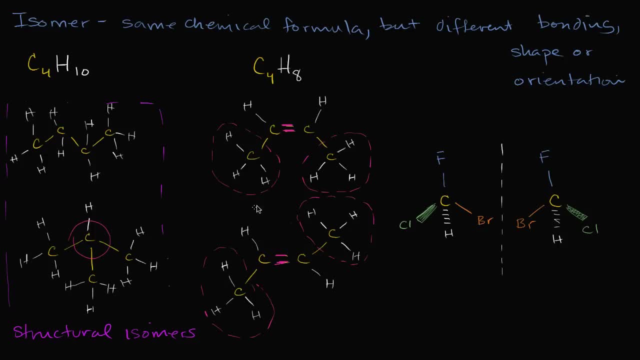 And so this type of isomerism where you have the same constituents and you even have the same bonding, this is called stereoisomerism. So over here we're caring much more about how things sit in three dimensions. 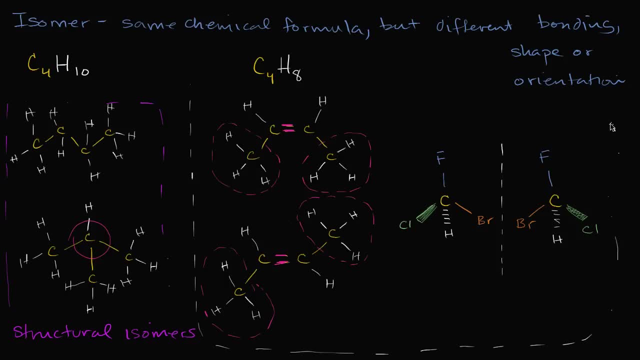 Not. we don't just care about what's bonded to what, or the constituents. And actually this one, as we'll see, this is also a stereoisomer, because this carbon is bonded to the same things in either case. So these are both. these are both situations. 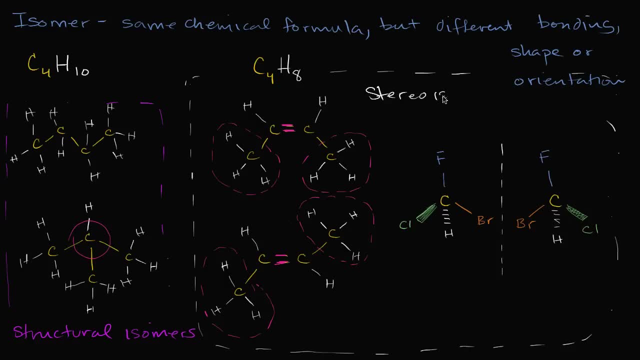 these are both stereoisomers, Stereo Stereoisomers, And this particular variation of stereoisomer is called a cis-trans isomer. Cis is when you have the two groups on the same side, Cis And trans is when you have the two groups. 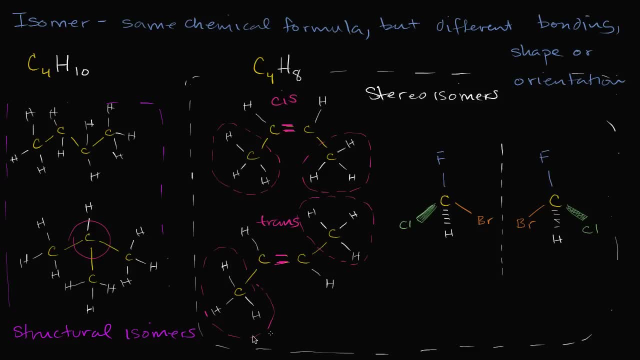 on the opposite sides of the double bonds: Cis-trans isomers, Cis-trans isomers, Isomers, And these are often called geometric isomers, Geometric, Geometric isomers, So that's a subset. So when I'm talking about cis-trans or geometric, 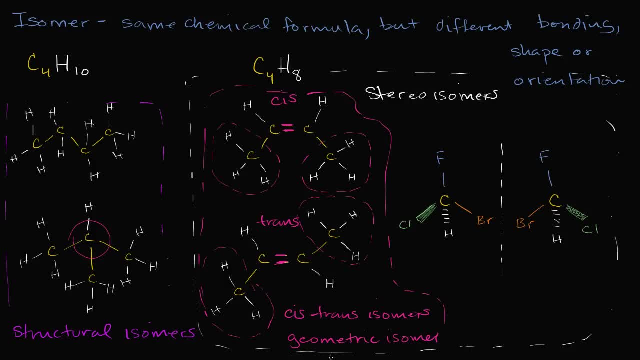 I'm talking about these two characters over here. They are a subset of stereoisomers. Now what's going on over here? I have no double bond. I'm not talking about cis and trans. The carbon, as I just said, is bonded to fluorine, chlorine, bromine and hydrogen. 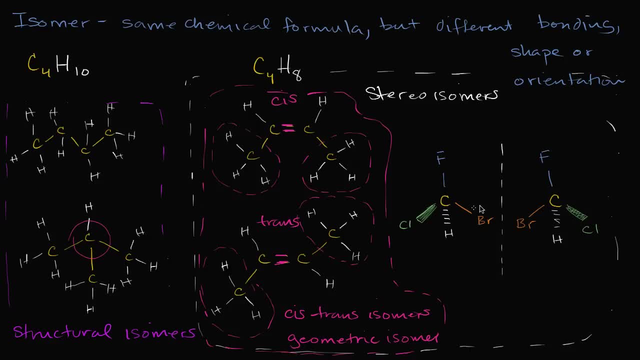 Fluorine, bromine, chlorine and hydrogen. How are these two things different? And the way that they're different is: if you were to actually try to superimpose them on each other, You will see that it is impossible. They are mirror images of each other.